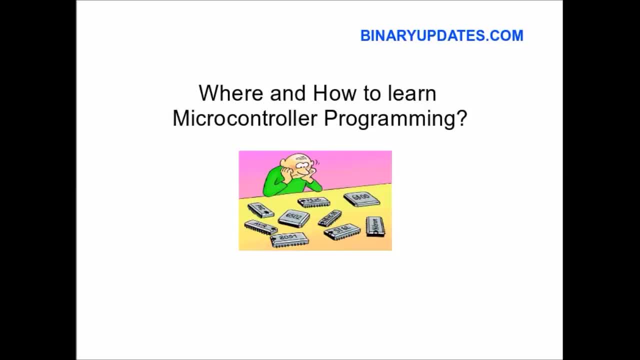 there are different microcontroller architecture available into the market. There are some examples, like we have AVR, we have a PIC from microchip and then we have ARM microcontrollers. So there are different variant that we have in microcontrollers like 8-bit and 32-bit. So for the beginners it's a big question where and how to get start. So let me give you a couple of tips which will help you to solve your question. So the tip number one is to choose any 8-bit. 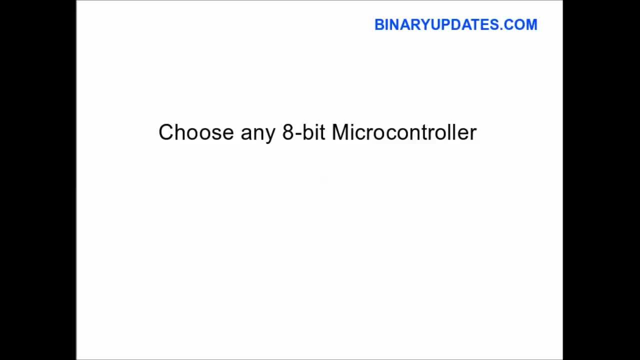 microcontroller. I say here 8-bit microcontroller, because you can even choose 32-bit microcontroller for the. but for the beginner, It's great to start with 8-bit microcontroller because it has a great amount of resources, free resources. we have tutorials available for that And they are. 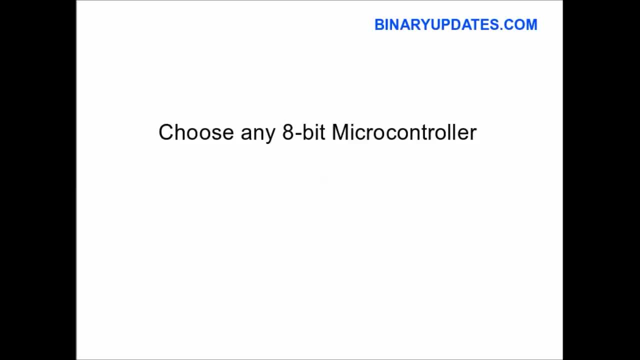 pretty explanatory and architecture itself is a little bit easy to understand at the beginner point of view. So you can choose any 8-bit microcontroller, and when you are a little bit confident about it, you can choose any 8-bit microcontroller, And when you are a little bit, 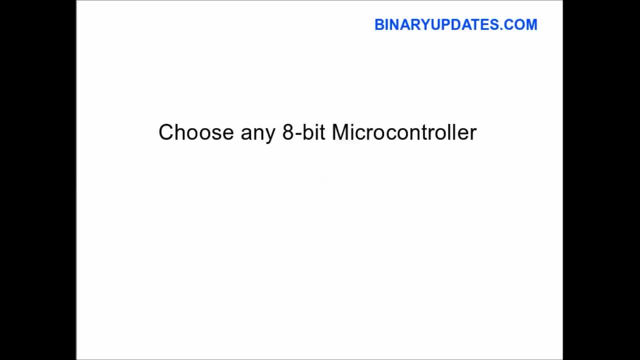 about 8-bit architecture. you can move on to 32-bit microcontrollers, So you have a couple of choices that you can make between 8-bit microcontrollers. Either you can choose 8051 microcontroller series or you can use AVR. AVR is something that I preferred all the time because it has extensive 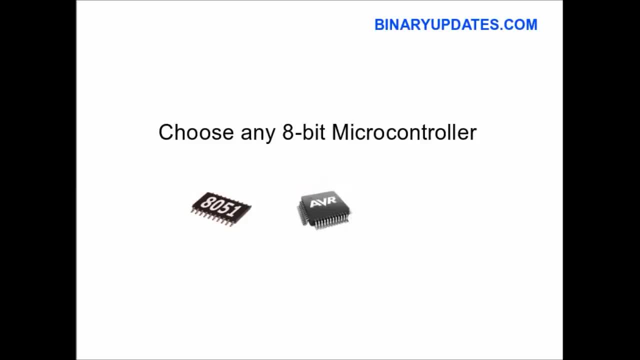 tutorials available on the web and there are a lot of user community support is there from AVR, So I choose to stay with AVR, But it's all up to you what you want to choose. You also have to choose a big microcontroller from microchip. It all depends on you what you feel comfortable with. Okay, so the first step is to 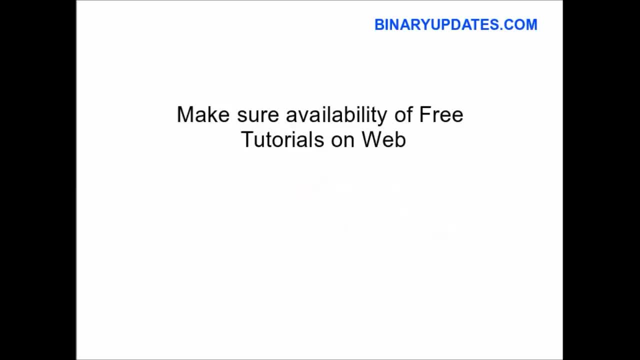 choose any 8-bit microcontroller Now. the second step is make sure availability of free tutorials on web, Because when you, when we are student and when we are a beginner, then we don't have enough money to spend to buy expensive books. We don't have enough money to spend to buy expensive books. 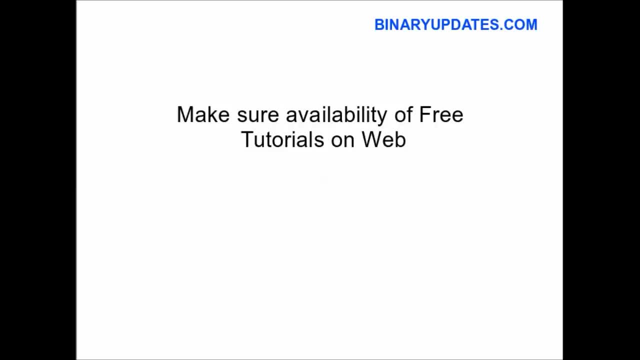 Or to go for expensive classes or training program which cost a lot and, unfortunately, student doesn't afford. Like me, when I was in the universities I was not afforded these things to do. So I recommend you to make sure the online free resources And, for example, especially for 8-bit. 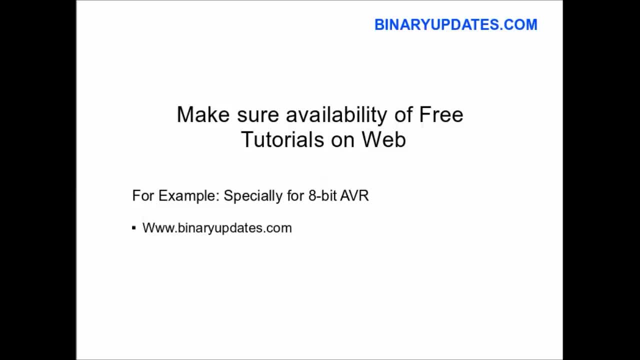 AVR. I will suggest you some of the websites. The first one is my own website that is a binary of webcom. Then there is another website: newbhackcom, maxembeddedcom, avrbreaknet and many more. So you can take a reference of this site and, you know, make your learning right smooth in the world. 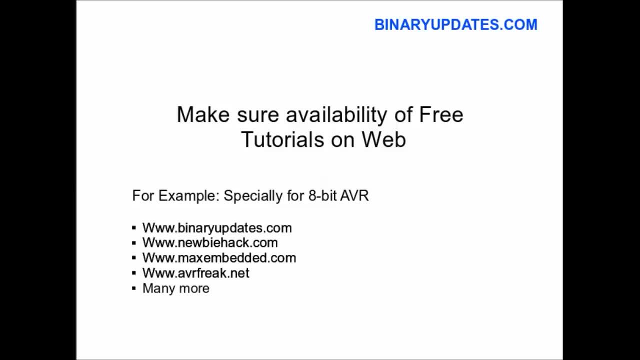 of microcontroller programming. Now the next step is to choose a right compiler and programmer. So what is compiler and what is programmer? So compiler, basically, is a programming environment- Sorry, it's a programming environment that we call compiler, And programmer is a piece of hardware. 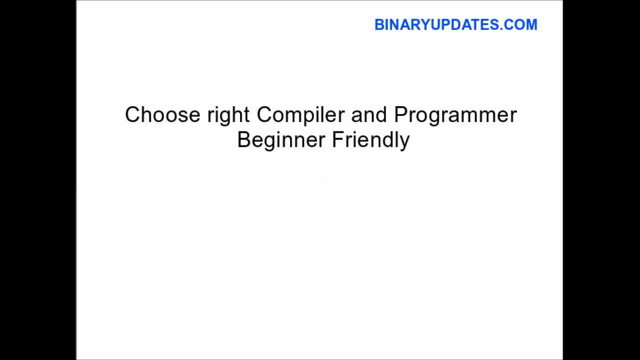 adapter which used to transfer your machine code- I mean the hex file- into the microcontroller. So it's basically program your code into the microchip. So when you start learning as a beginner you have to make sure that you choose a right compiler and right programming adapter. 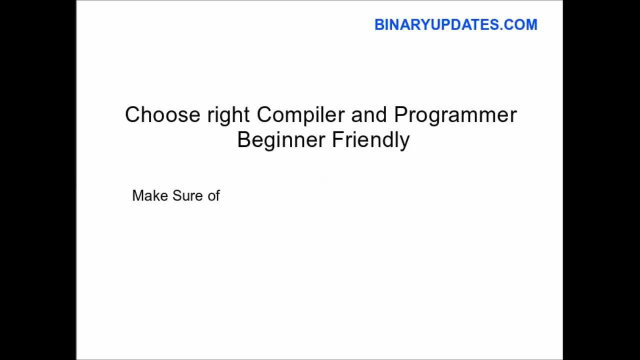 There are a couple of things you have to make sure before you choose and start experiment with your compiler and programmer. The first point is to make sure that the good documentation available in terms of user manual, Because when you are new, you always have to take a reference of user manual when you 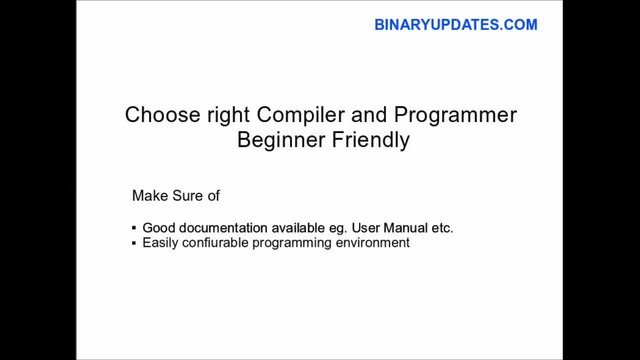 write your software for your microchip. The second thing is you have to make sure that your programming environment, that is, your compiler and your hardware programming adapter, is easily configurable in the beginner point of view, Because you don't have to spend a lot of time. 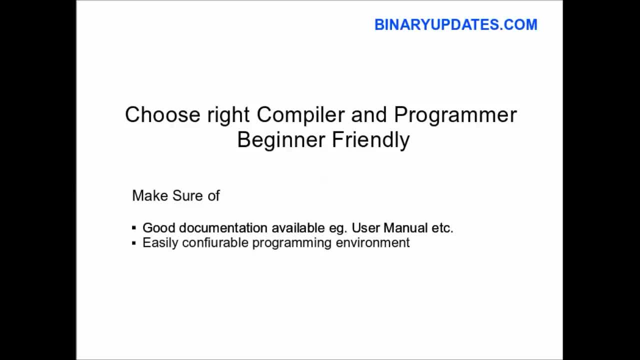 to configure your software and hardware instead of focusing on programming. So I recommend you to make sure that you choose the right programming environment and hardware adapter. Then the next point is to make sure the compatibility with your operating system, Because in today's world we have a lot of different operating systems from Windows. 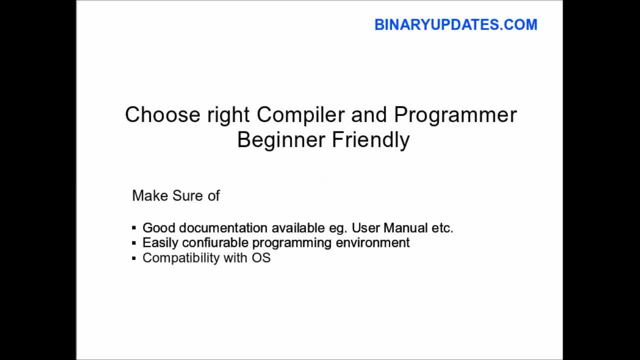 Linux and Mac And in Linux itself we have a different distribution of operating systems. So if you are a kind of person who make a lot of experiments with your computer, with your system, and try a different operating system, then you have to make. 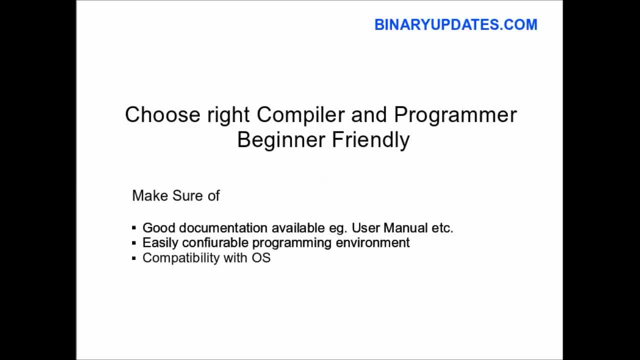 sure that your programming environment and your hardware programming adapter is compatible with your operating system. And the next thing you have to take care, which is very important in terms of embedded developers- you have to make sure that your programming environment- I mean your compiler or maybe your programming adapter hardware adapter- has a great simulation and 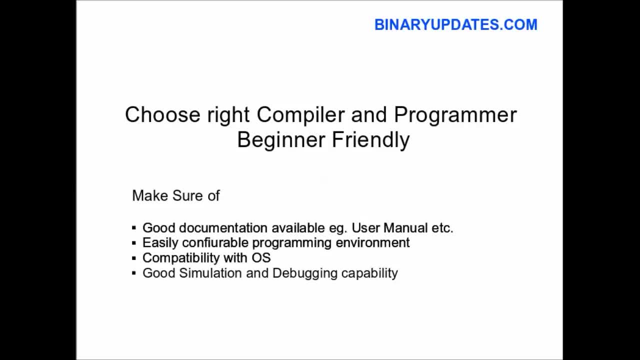 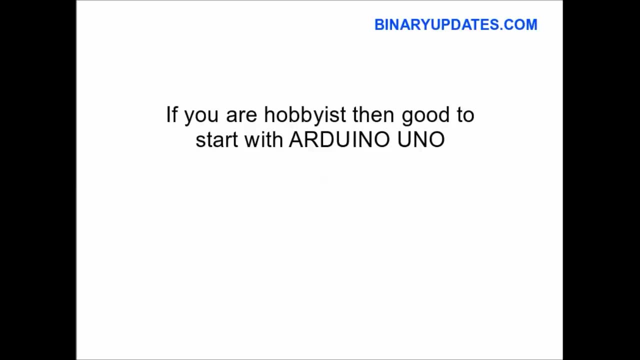 debugging capability. This is the one thing that you have to do over and over again, and you have to have the expertise to become a good embedded developer. So you have to make sure this couple of things. And the next tip I want to give you if you are a hobbyist, and if you are a hobbyist- 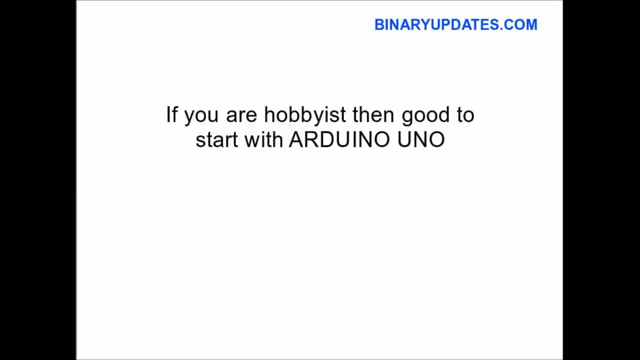 or student, and if you're very, very new and you don't want to get into the startup world, then I would recommend you to use Arduino Uno hardware adapter. So this is a little interesting board that's been designed by Arduino Incorporation. It's a company in Italy. 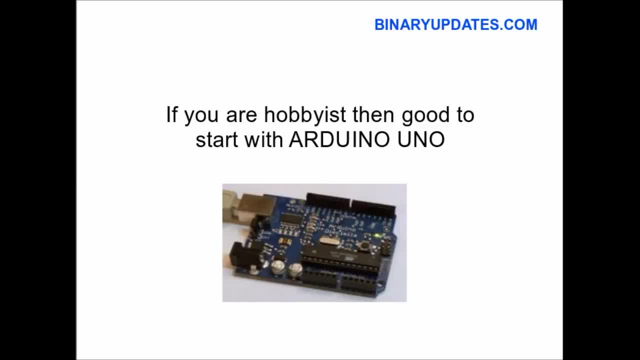 I don't know how to pronounce this name, but I think I'm right- Arduino And you can use this, this kit, which is very easy to use and has a lot of tons of different examples, Tutorial available on Google, on YouTube, and it will be very easy to get started with this. 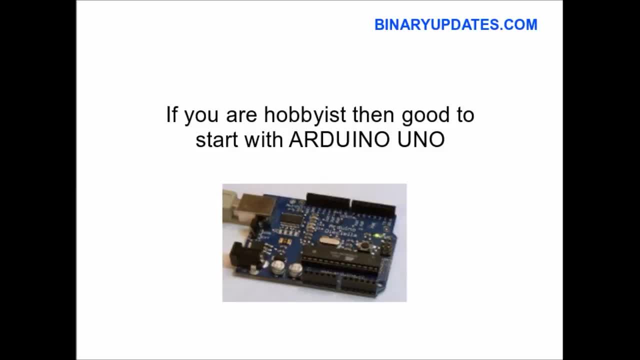 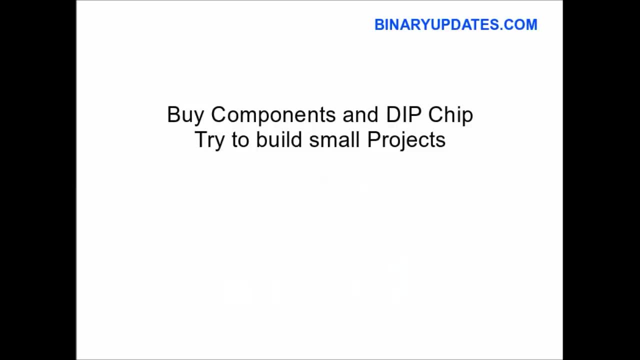 Just Google with its name and tutorial Arduino Uno tutorials or something like that, and you would get tons of things to get started. And the next step is very important, as in electronics and embedded developer point of view: Buy your own components. you know, just go to a retail shop and buy your own components. 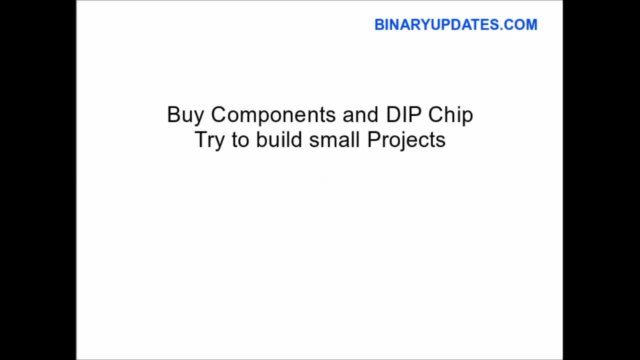 preferably buy DIP chips And you may use some kind of some kind of breadboard circuit and put your microchip into the breadboard and try to build small little projects. And if you don't really have a time to you know work around electronics, then you can even choose something like this: 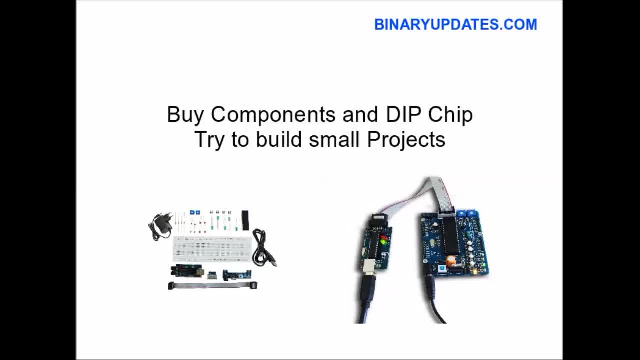 What I have shown you here. it's a beautiful kit designed by Tinker Sky Electronics, and they made a hardware programming adapter for AVR chip. This is just an example I'm going to take in terms of AVR, but you can have a lot of different products available into market that you 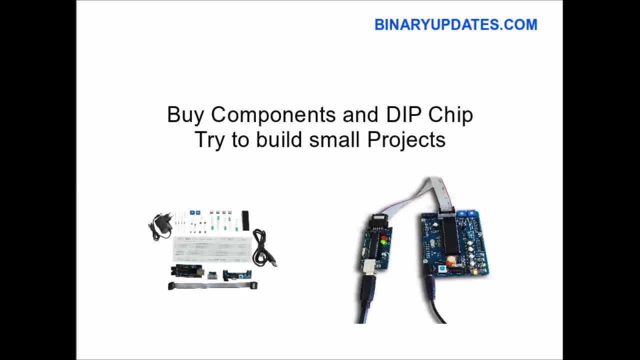 can make use of. So it's very important to buy your own components, your own adapters, and you know learning by doing is the best approach to learn microcontroller programming. So I recommend you to go with that and buy components and do by your own. 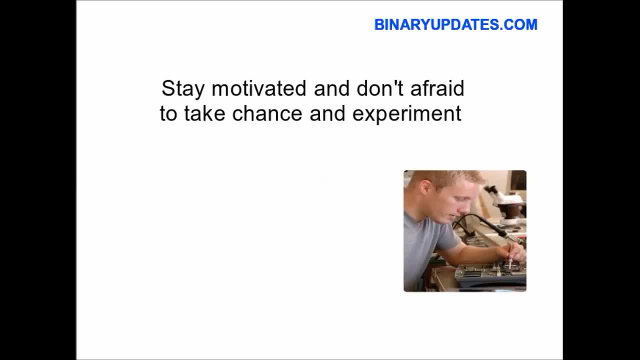 The next step is. the next thing that you have to do is you have to be always stay motivated and I recommend you don't be afraid to take chances and make experiment with your sockets, with your microcontroller chip, to write different interfaces, and make experiments to check the things, how things work, and I mean to 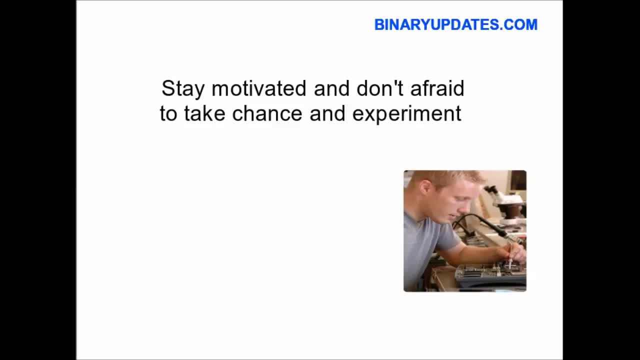 understand how electronics work. so this is very important because you will be finding in trouble working on the problems and errors for several hours or several days. so in that case you have to be. don't just give up when you are beginner because you have to embedded system or a microcontroller programming. 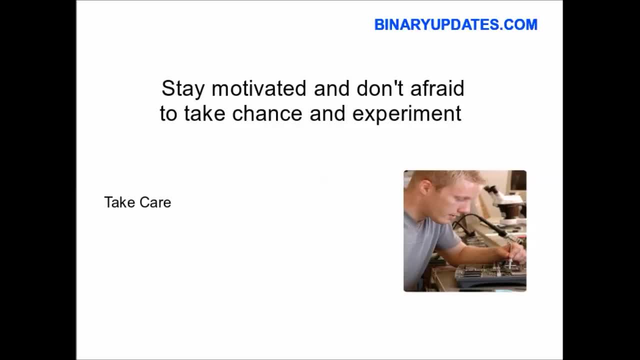 needs to have a steepest learning curve. it's not a something, it's not a learning process that you can achieve it for one day or one month or something. it has a very steepest curve. you need a time and patience to learn and you always need. 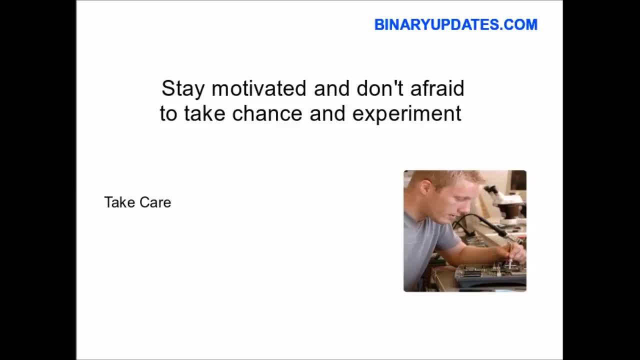 motivations to learn. so a couple of things you need to take care when you are start your experimenting with a microcontroller chip. you have to take care of input voltage. if you exceed input voltage then the power rating of your chip, then you will find your chip will burn out and you will find in 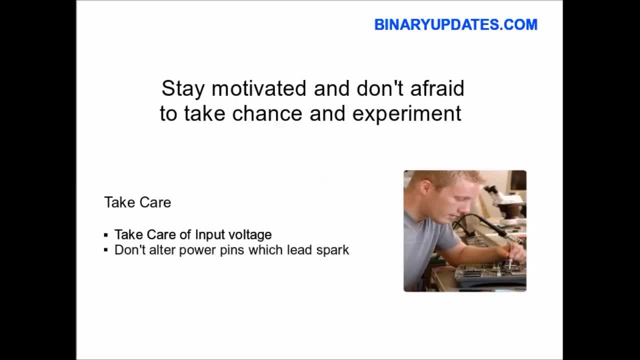 troublesome situations. the next thing you have to take care is don't alter your power pins, because if you alter your VCC and a ground it will lead the spark and you will again find your chip will be burn and your circuit will be short. and I just want to make, I just want to recommend you to keep multimeter with you. 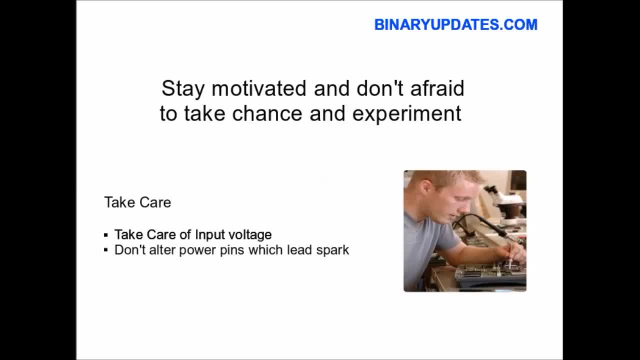 and keep, keep dragging your voltage and keep making sure that your power pins which one is VCC and which one is ground". the next two steps which actually give no requests to the happening of the energy. I said once, and the next thing I have to say is be careful before water retention is happening, while you are. 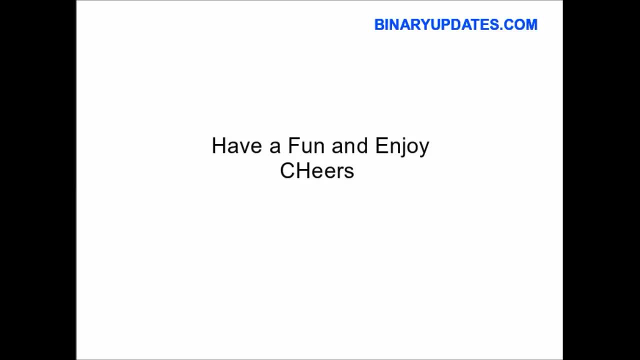 working with a multi meter chip message and you also have to make sure your bypass� will not be, not you worry about thermal voltage if you don't have. at this point, and I just want to make, I just want to recommend you to keep multi meter with you and